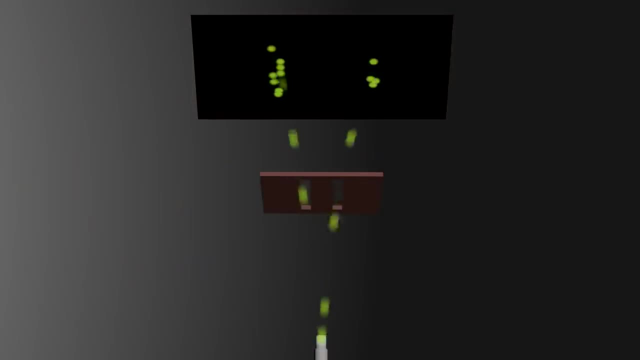 tennis balls and throw it at a double-slit, Will I see the same kind of behavior that electrons or atoms have? No, of course not. I'll just see two patterns on the back wall. Why doesn't this thing behave like electrons or atoms? It's made up of atoms and electrons. 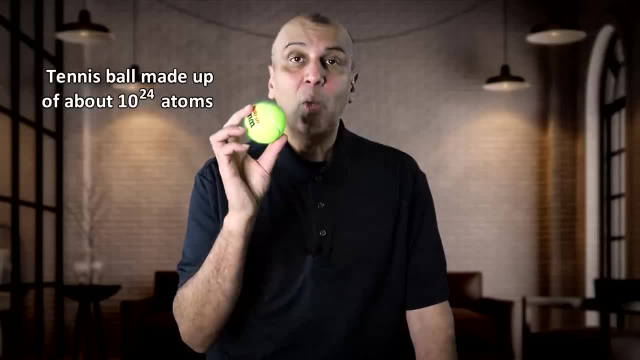 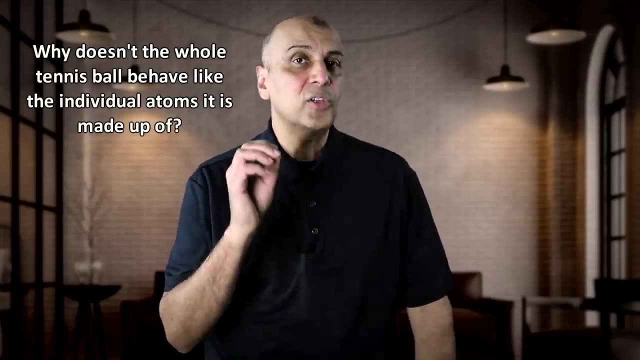 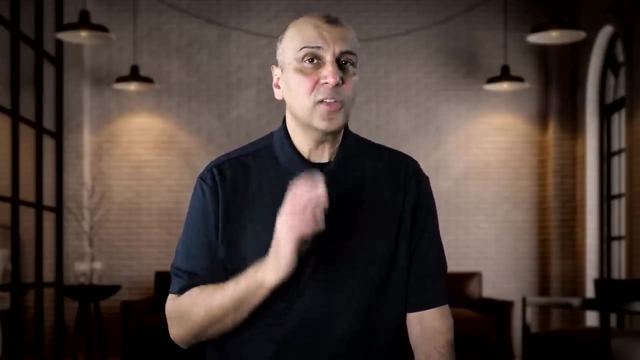 around it six trillion trillion atoms. Why doesn't the whole behave like the individual particles it's made up of? To answer this, we have to understand some of the basics of quantum mechanics. Let's look at how the double-slit experiment works with light. first, The results. 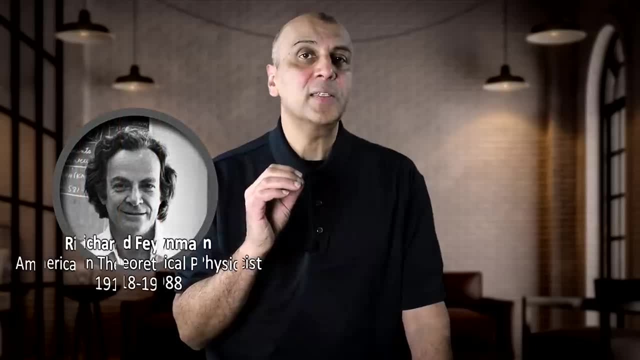 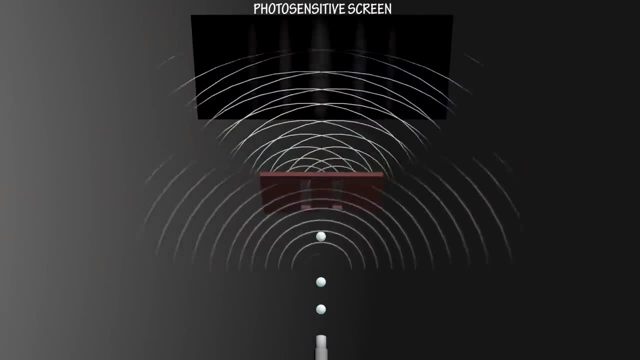 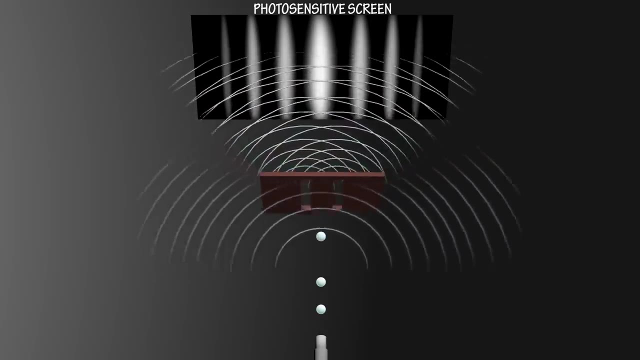 are the same with electrons or atoms. Richard Feynman called this the central mystery of quantum mechanics. When we shine a monochromatic light that is light of only one wavelength through two slits as light hits the screen, we see an interference pattern on the other side because, as the 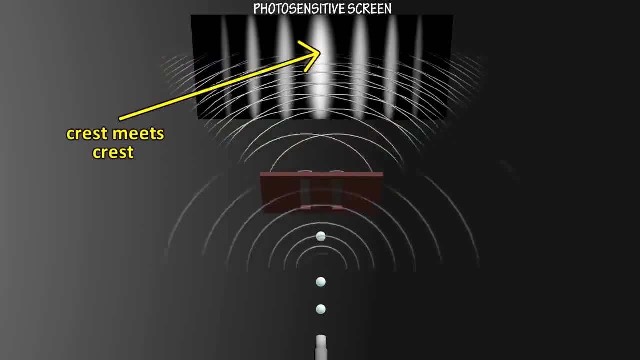 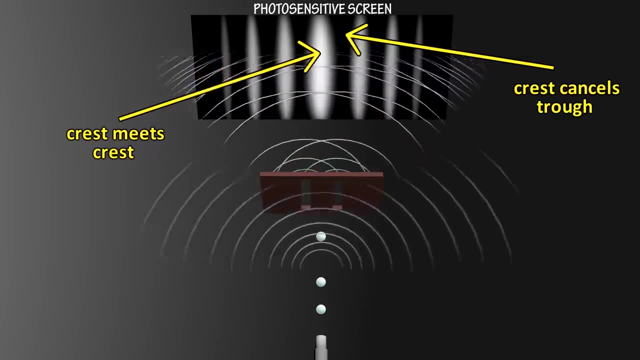 waves spread out. the crest of one wave hits the crest of another, It becomes stronger. Where a crest hits a trough, it will cancel. This should be no big mystery. This is not quantum mechanics. This is just a property of waves. It'll happen with water waves too. 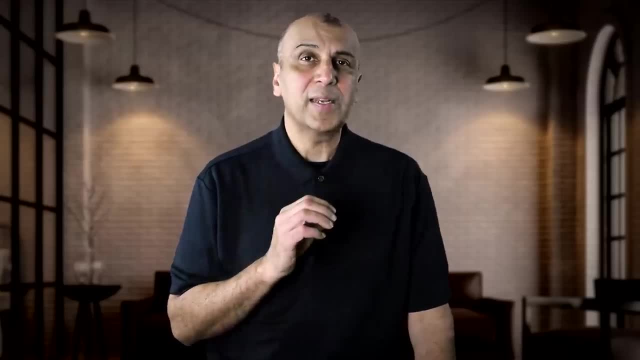 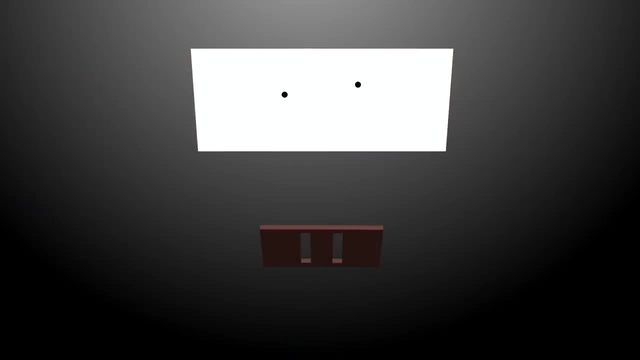 Now what if we lower the intensity of the light and keep the intensity of the light lower until our light source emits only one photon at a time? Surely this should not create a wave pattern. When we shoot one photon at a time, it forms a dot on the screen, But 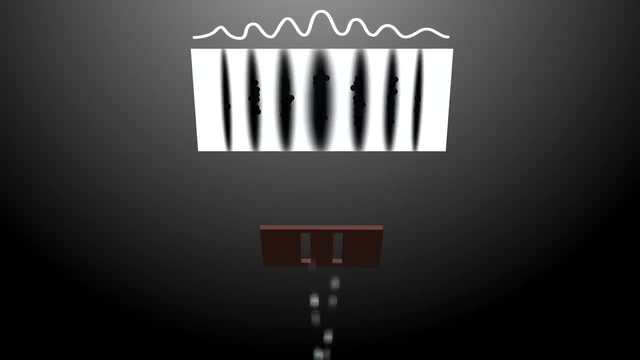 if you fire enough of them, thousands or millions of photons, what you find is that collectively the photons form the same interference pattern. So somehow the photon either interacts with itself or somehow is able to communicate its part in the interference pattern when fired one at a time. 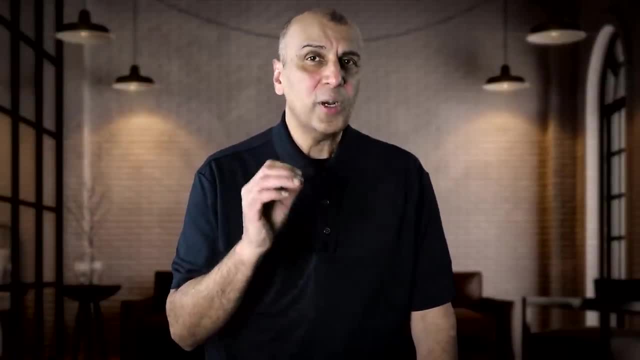 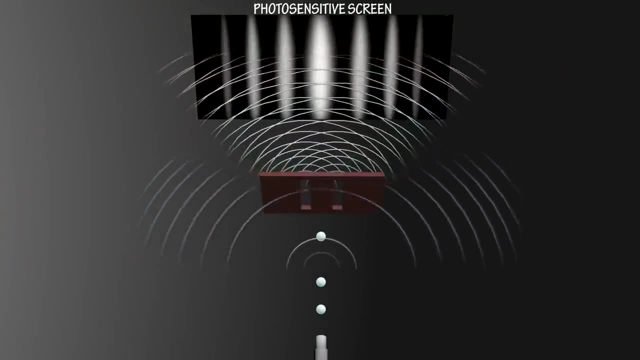 So, since we want to find out what happens when we shoot one photon at a time, let's find out what's going on at the slits. What if we put a detector there to determine whether the photon goes through slit 1 or slit 2? This is the most startling result of quantum. 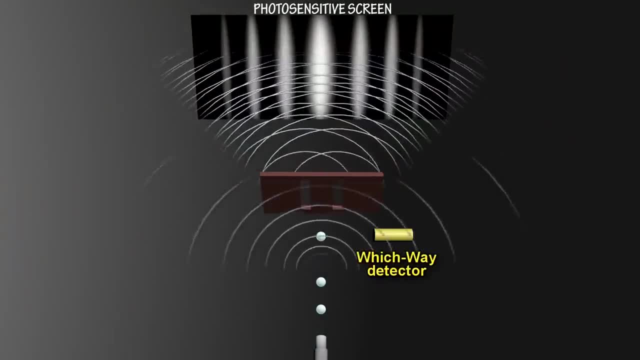 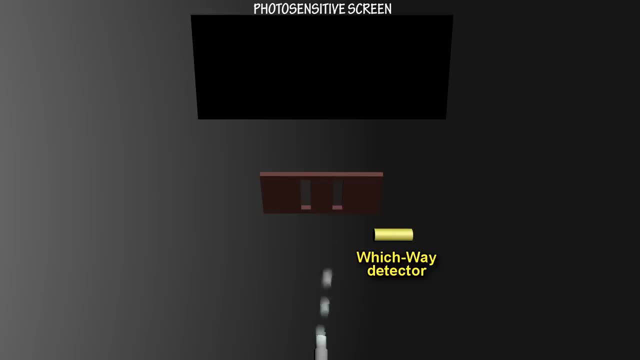 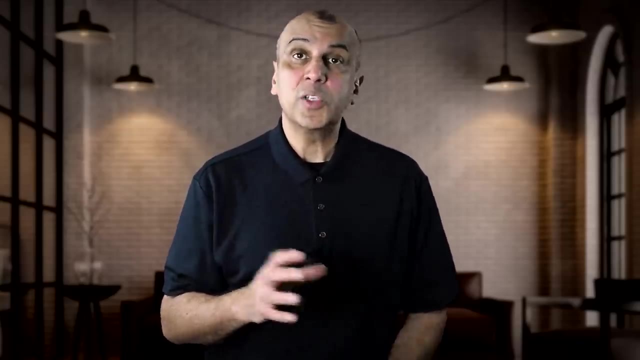 mechanics, because when you try to find out which path the photon took, the interference pattern disappears. The photon appears to now behave like a particle instead of a wave. So what's going on? Let's talk in the language of the Copenhagen interpretation, which is: 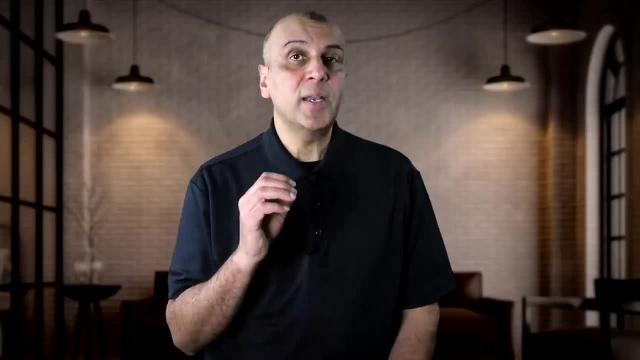 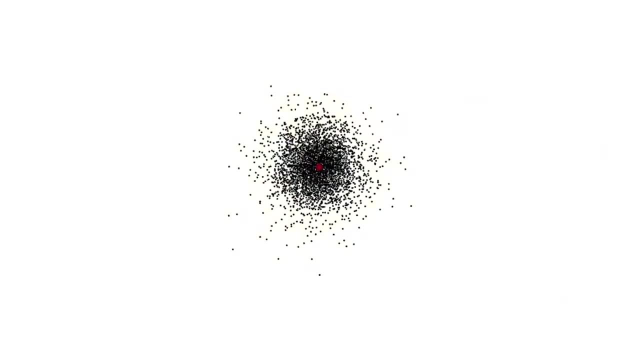 the most accepted interpretation of quantum mechanics. What's going on? Let's talk in the language of the Copenhagen interpretation, which is the most accepted interpretation of quantum mechanics. This was conceived by Niels Bohr and Werner Heisenberg at the University of Copenhagen around 1927. This interpretation basically says that these so-called 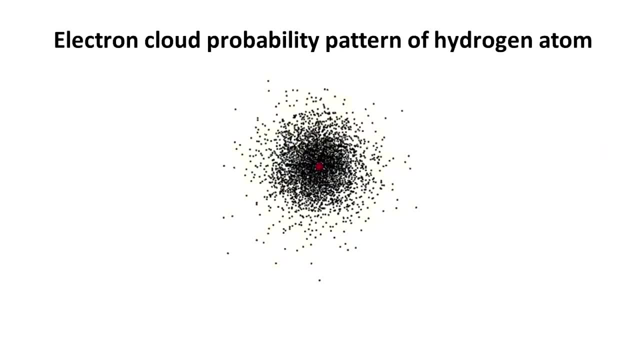 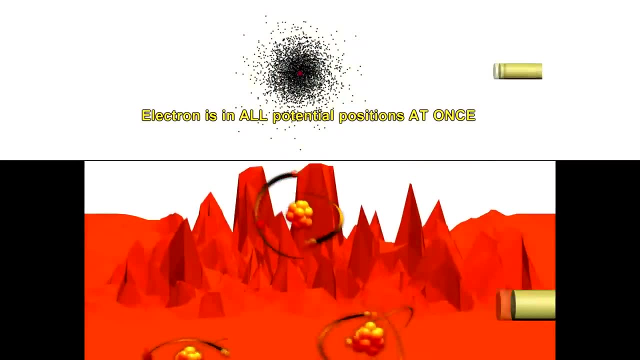 particles are not particles at all, but really like clouds: They are in multiple states at the same time. They are like waves of probabilities. The waves become distinct like particles only when they are measured At the point at which the probability wave becomes a distinct particle. 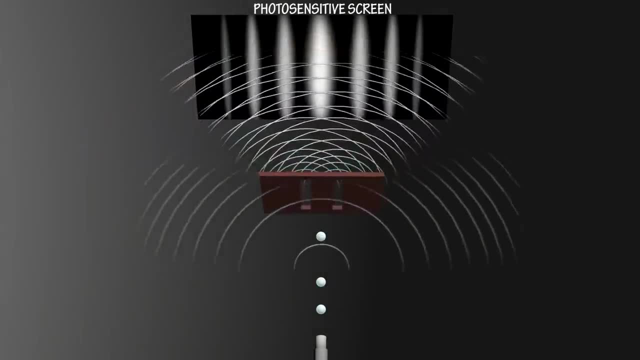 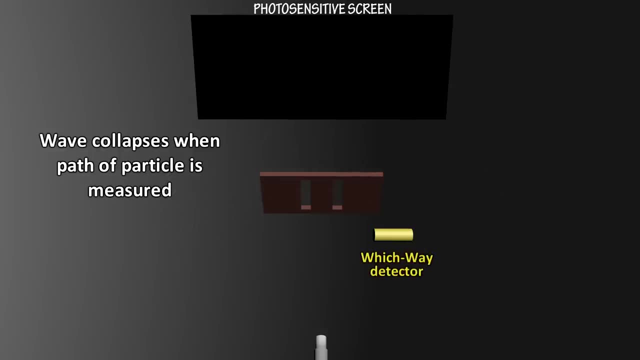 is called a collapse of the probability wave. What scientists have found is that, at any point when the which path information – any particle is measured – its probability wave collapses, For the particles to remain probability waves, their path information must remain in absolute secrecy. 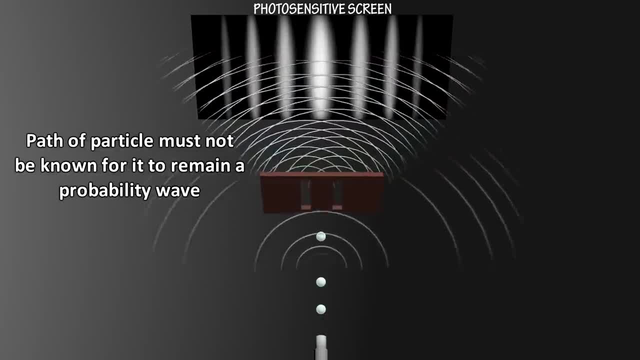 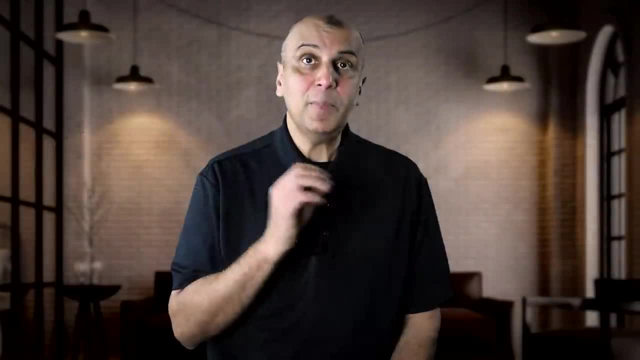 If, at any point, any kind of measurement is made, whether it is seen by anyone or not, the particles become distinct and do not display wave-like behavior. This same behavior has been found in subsequent years with electrons in most other states of space, For example. 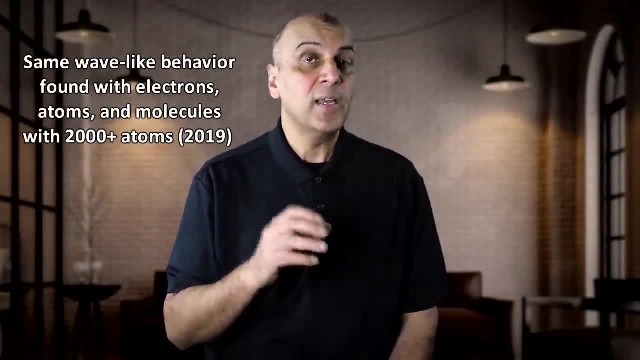 these are well-known wave-like particles. This is a proof that they are not wave-like. The same behavior has been found in subsequent years with electrons and electrons, The difference atoms and even molecules composed of as many as 800 atoms. The same interference pattern forms. 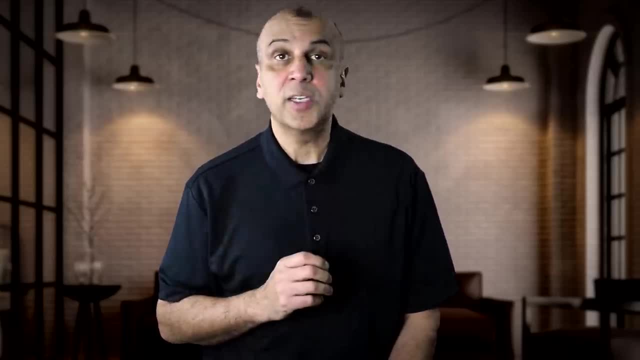 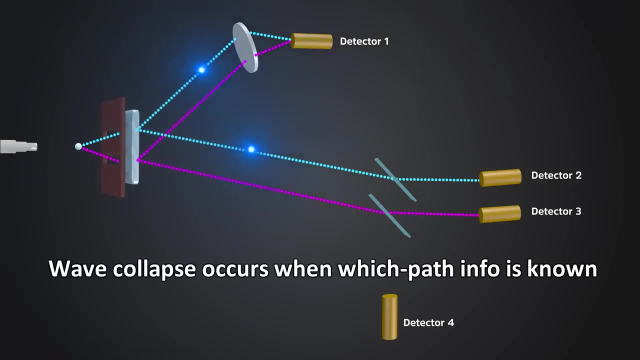 and the same collapse occurs if their witch path information is measured. A measurement, always collapses the wave. So what is a measurement? A measurement is a formation of any physical record of which path the particle takes. It's not about conscious observers, It's 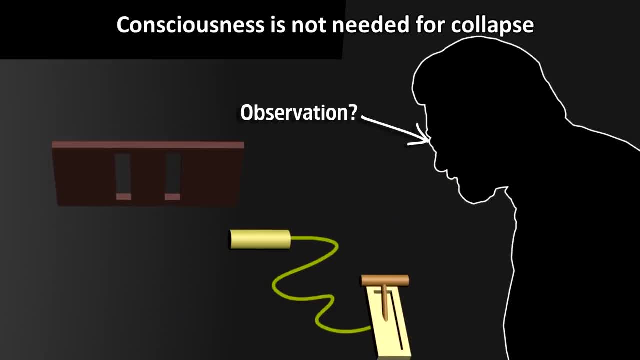 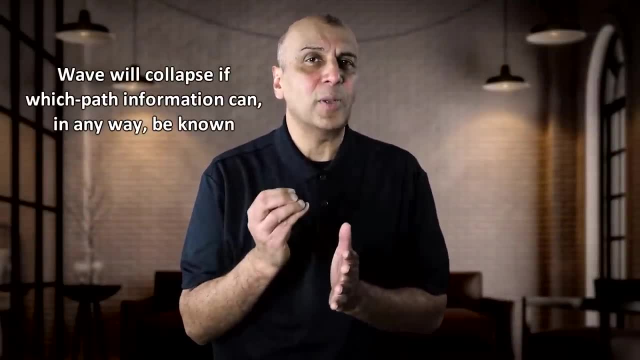 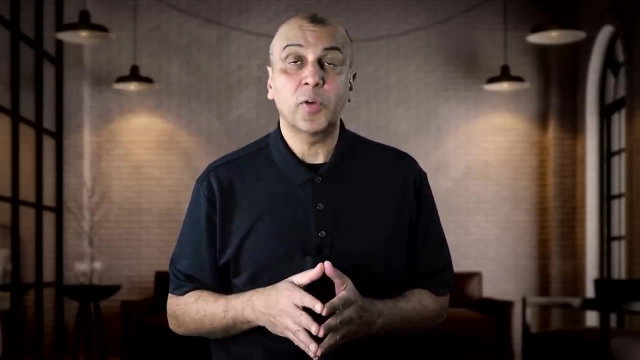 about a record made in the universe, even if no one is looking. It is such that a forensic exam, if we had even the most sensitive quantum tools, could establish which path the particle took. You never have to look at the information. You can even destroy the information before you look. 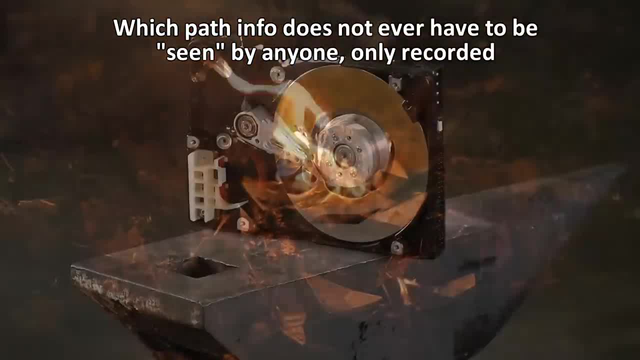 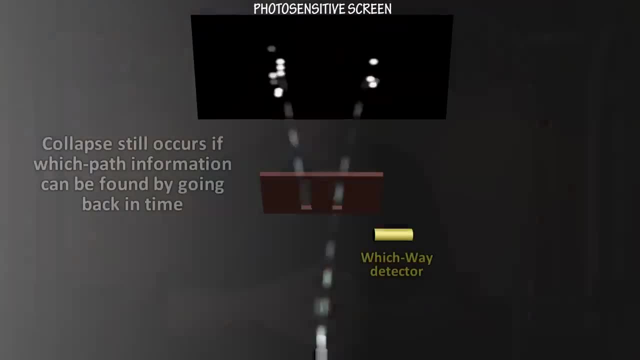 at it like burn it or destroy the hard drive that it's on, The wave will still collapse because the universe already recorded it. Why is it recorded, even if you destroyed it? Because, theoretically, the wave will still collapse even if you destroyed it. 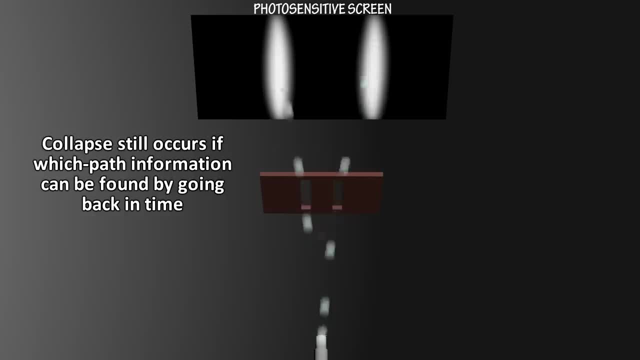 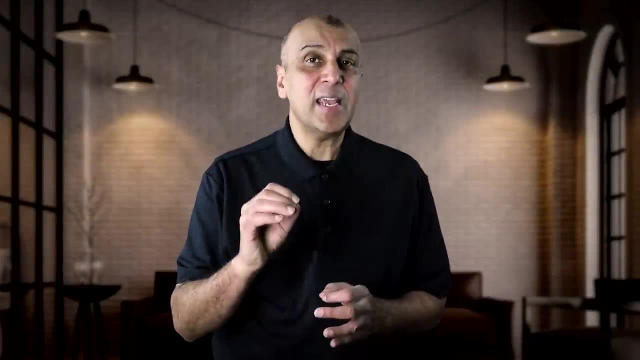 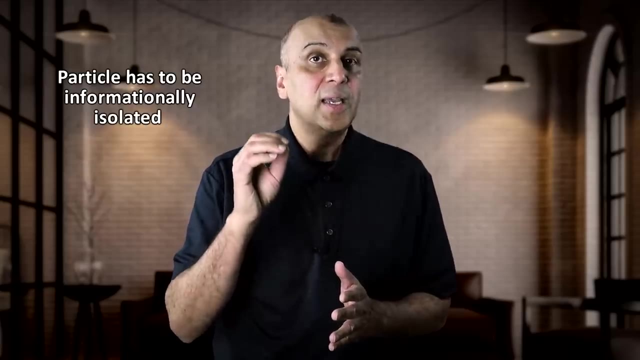 You could go back in time and see the path. The universe will say, hey, I already know the path. Now it's a particle, You can't have your wave back. The path has to be taken in absolute secrecy. The particle has to be informationally isolated. The interference can only occur. 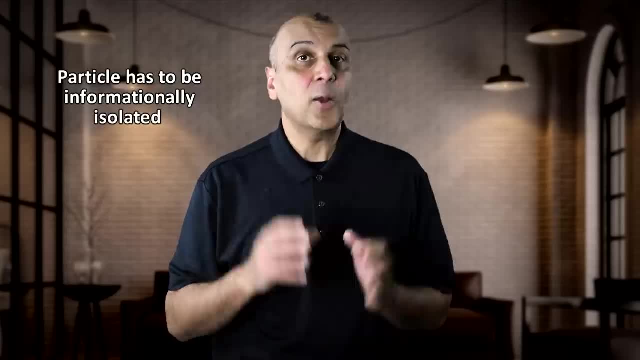 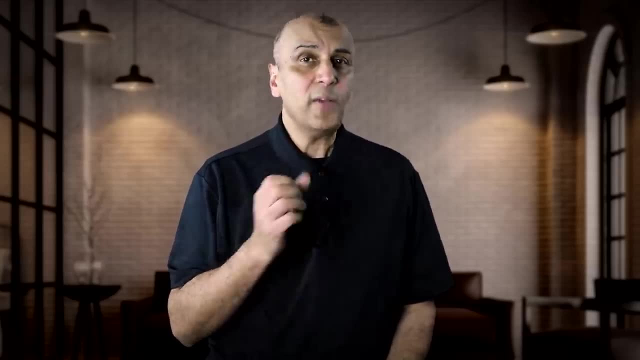 if it is impossible, even in principle, to find out which path the particle took? Now, as I said, this happens with photons, electrons, atoms and even large molecules. Now, what if we do this? What if we do this with really large particles like grains of sand- which, by the way, 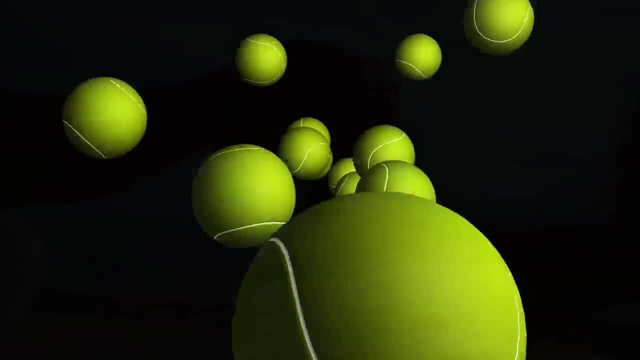 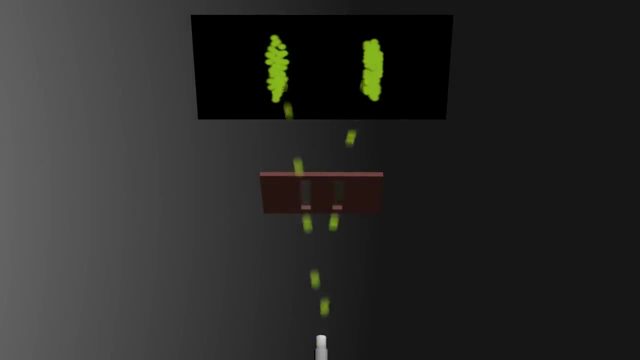 are typically composed of quintillions of atoms, or tennis balls. Will we see the same pattern? Of course not. We'll just see two lines on the other side of the double slit. Why don't we see this behavior with tennis balls? The reason is that large objects are nearly 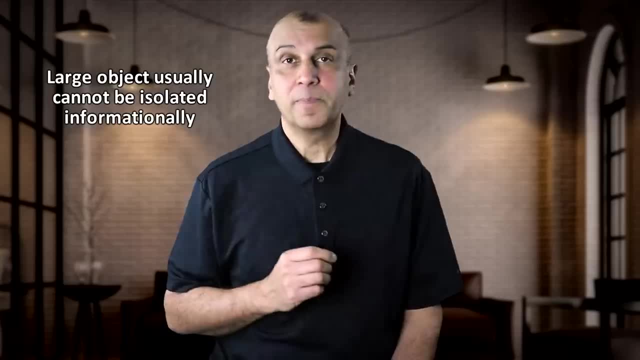 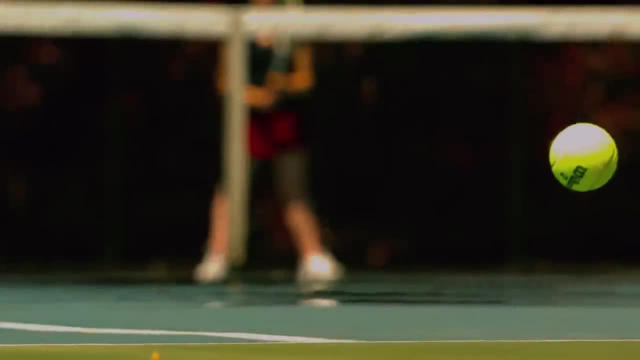 impossible to isolate informationally from the outside world. What do I mean by this? Let's look and see what it would take to isolate a tennis ball. Remember, to do this, we have to make sure that there is no record made anywhere in the universe. 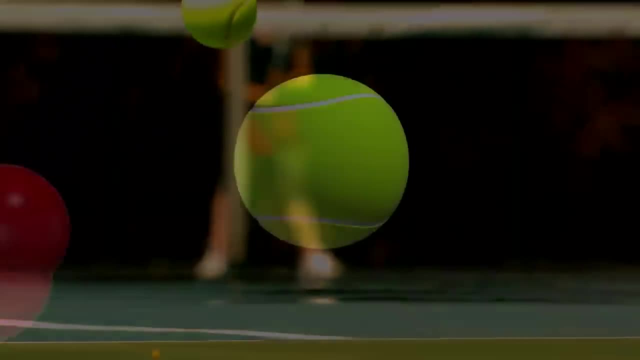 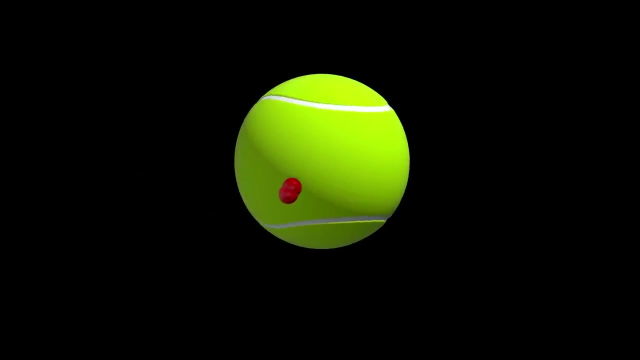 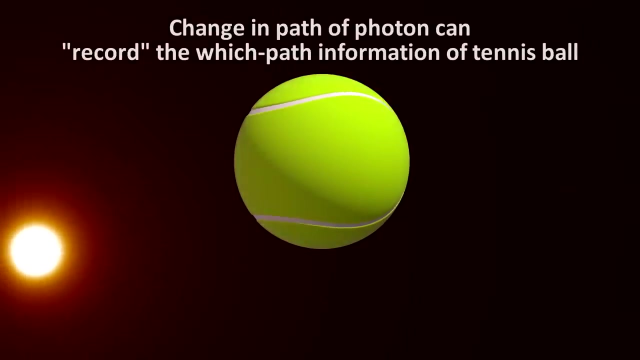 of which path the tennis ball follows. First we have to remove all the air and photons in the experiment. Why? If a photon or air molecule bounces off the tennis ball, then it has potentially recorded the path of the tennis ball. For example, if the photon reflects off the ball. 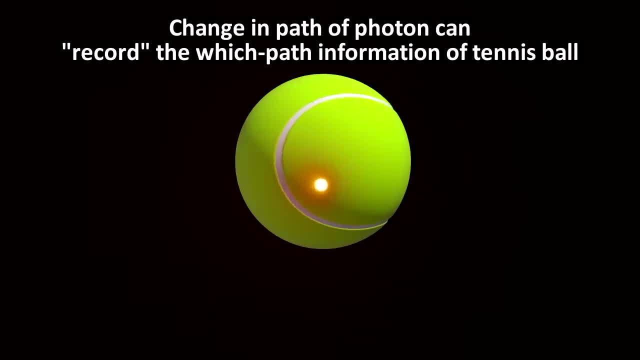 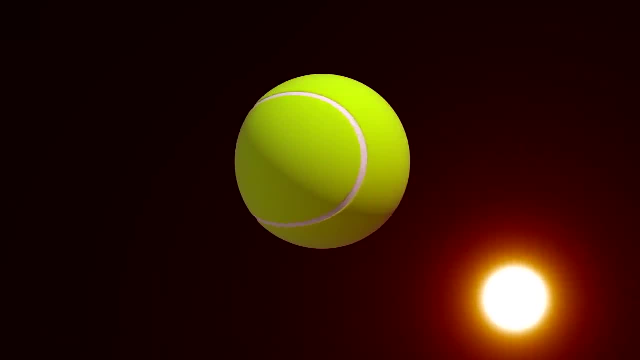 then that could be a measurement, because the path of the photon would be changed and the bounced path of the photon has recorded the path information of the ball. Potentially, someone or the universe could examine the paths of all the photons in the room. 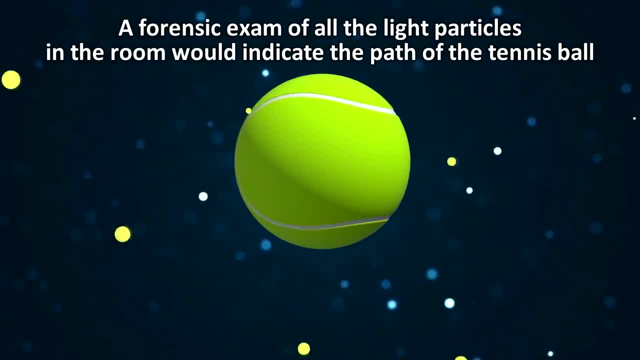 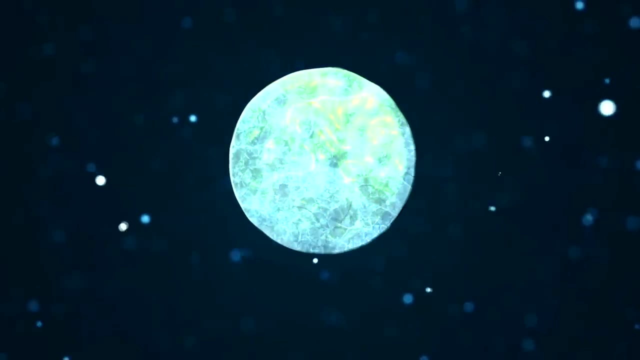 find out how they were affected by the path of the tennis ball and find out from that information the path that the tennis ball took, And the same thing applies for atoms. We'll also need to cool down the temperature of the ball to near absolute zero, because a ball that has any temperature will. 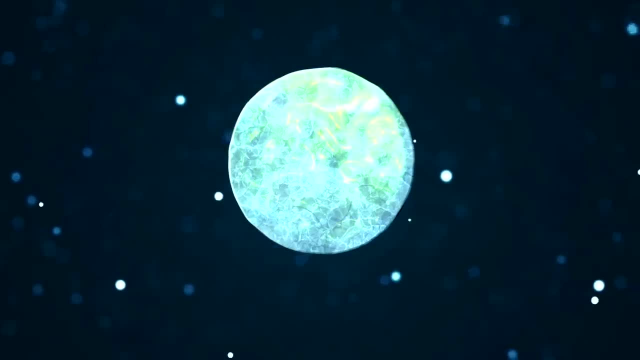 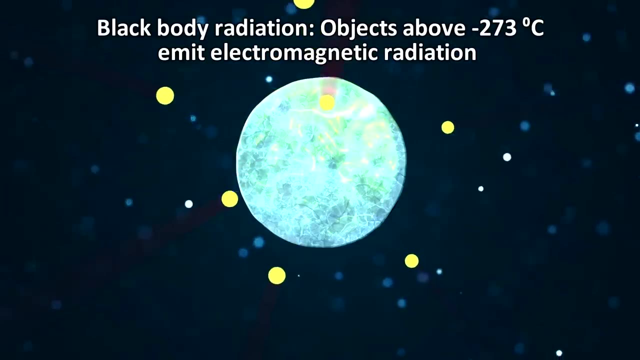 emit photons due to something called black body radiation. This is a property of all bodies with the temperature above absolute zero, which is, by the way, negative 273 degrees Celsius. The emitted photons will have recorded the information about the tennis ball, such that someone examining the 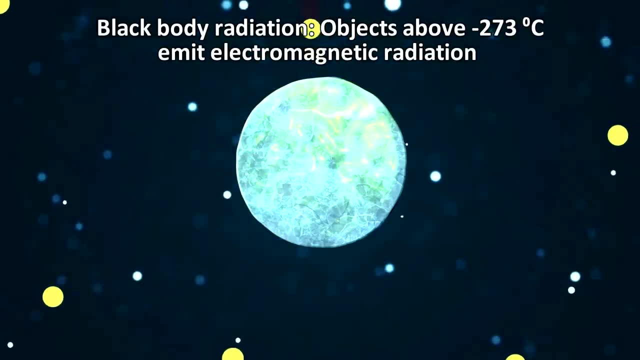 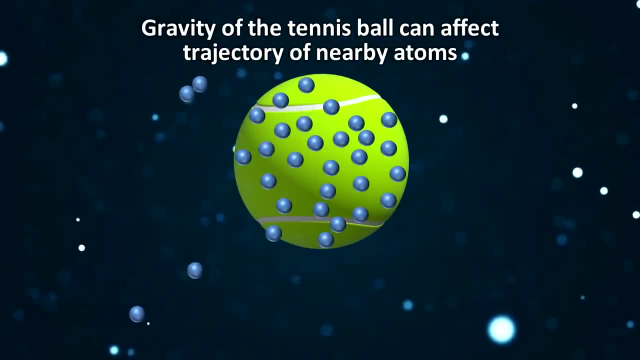 photons in the room could determine the path of this tennis ball. We even have to worry about the gravitation that the tennis ball will have. Why? Because this gravitation of the tennis ball will affect nearby atoms. This, in principle, can allow someone to determine the path that this 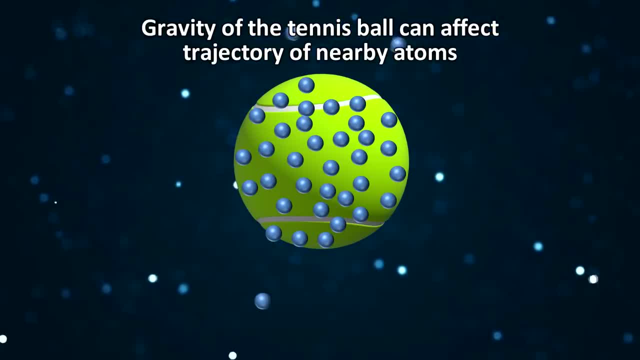 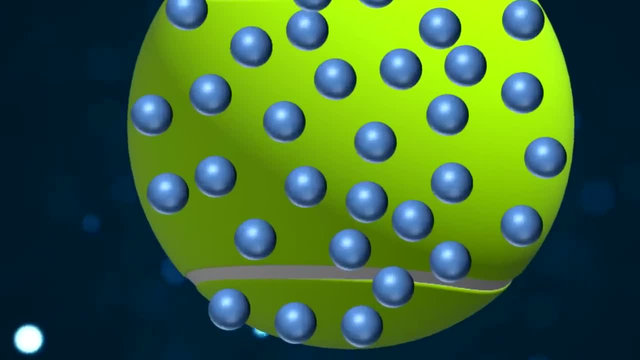 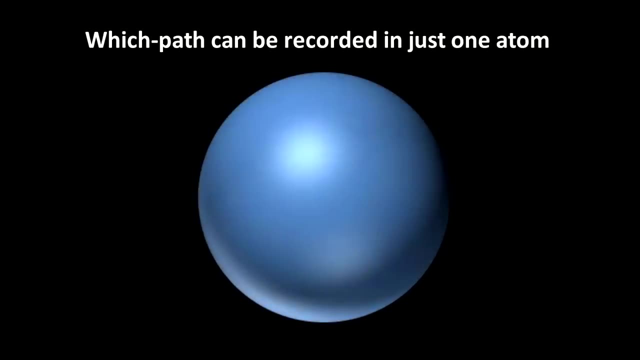 tennis ball took. The movements of nearby atoms can also form a record of the path of that tennis ball. We have to completely isolate the tennis ball because any information that is leaked to the universe about its path will create a record, even if this information is recorded in one atom. 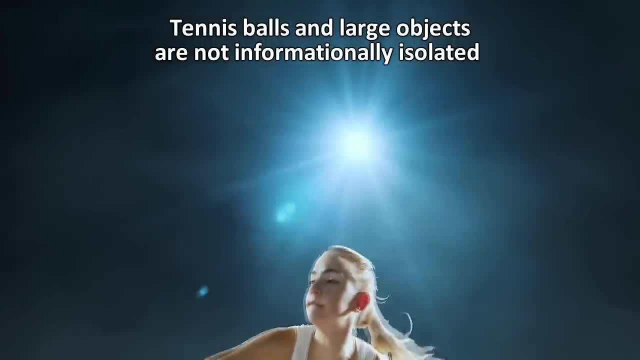 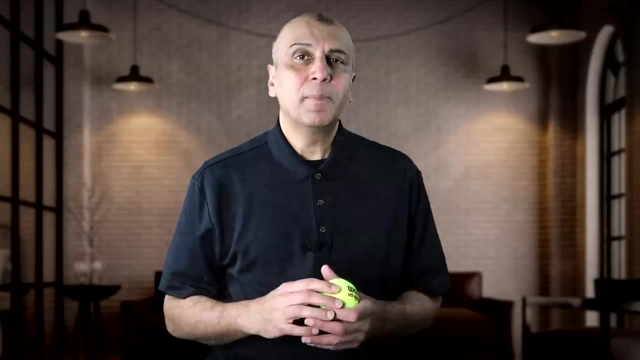 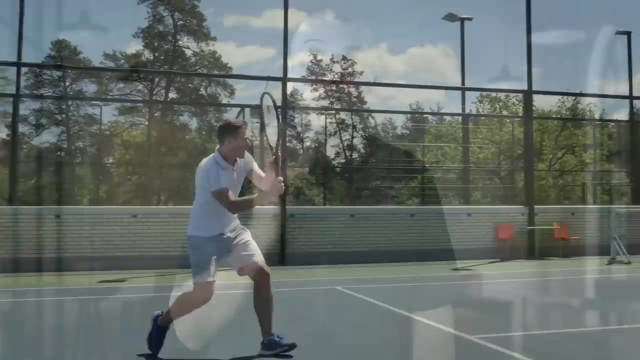 It is still information which has been captured in the universe. And the tennis ball will not be superposition. It will not be a cloud, It will be a distinct entity. Macroscopic objects like this are very difficult, if not impossible, to isolate informationally. So in our everyday experience, 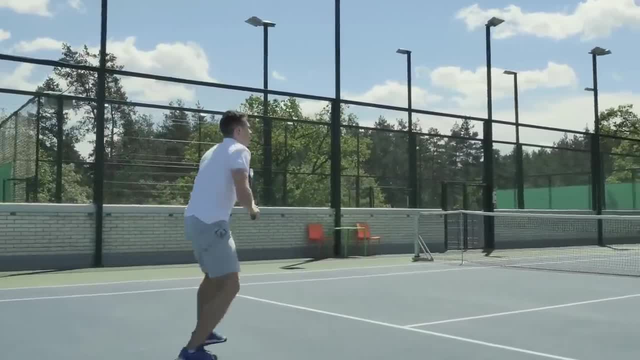 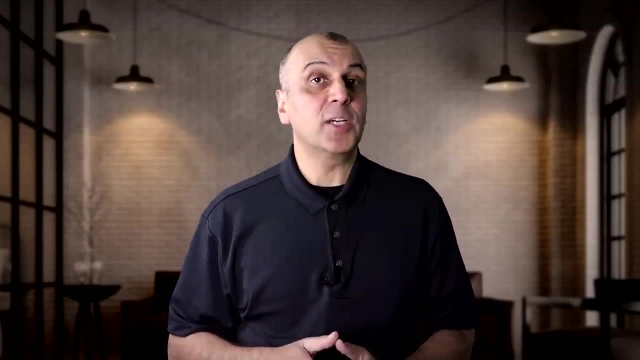 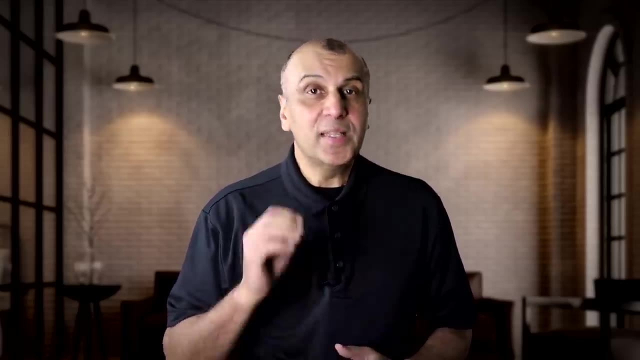 we will not see quantum superposition or wave-like behavior of macro objects, But one principle of quantum mechanics is that it applies to all objects, regardless of size. Could the tennis ball behave like an atom if we could isolate it informationally? This may be true, but there is a measurement problem. We can look at this. 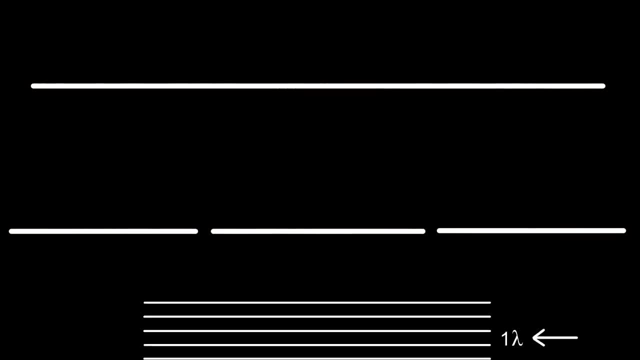 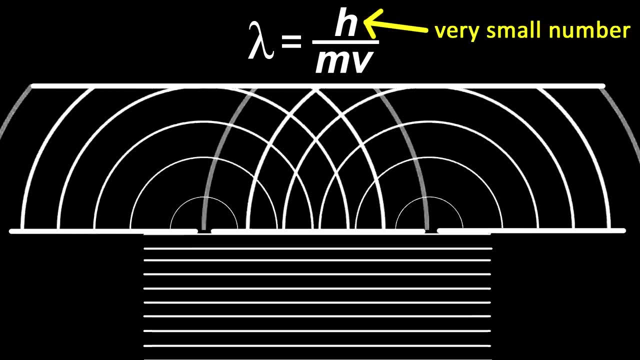 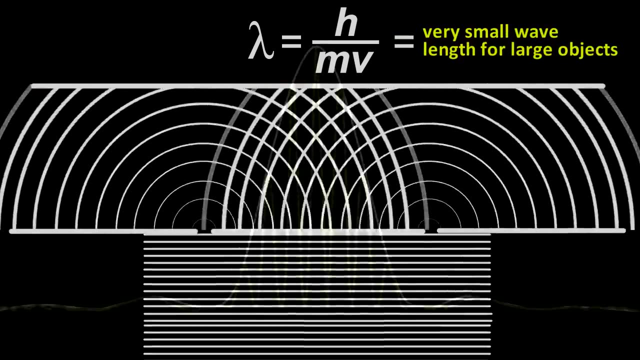 mathematically, The wave of an object is described by the de Broglie wave function. Lambda equals Planck's constant over mass times velocity. Since the Planck constant is so tiny and the mass m so huge, the wavelength will be extremely small. So the interference pattern, for all intents and 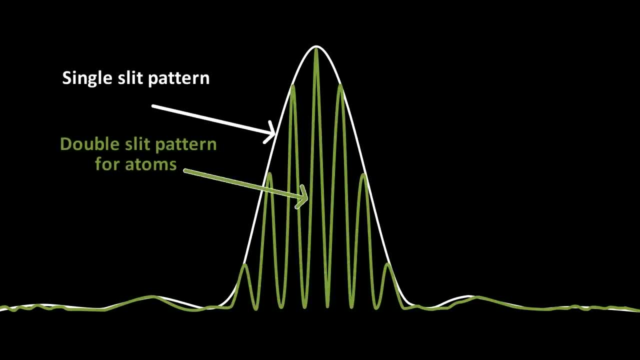 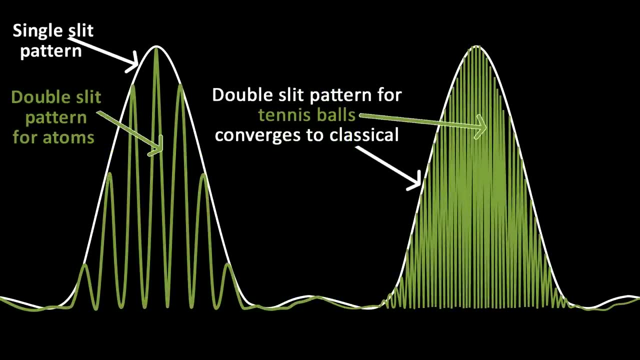 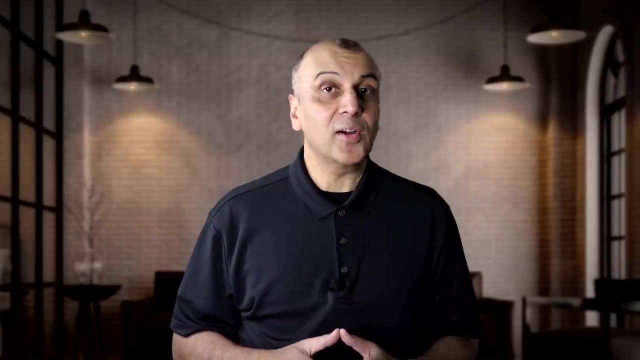 purposes will be no interference. The quantum mechanical behavior of the tennis balls converges to classical behavior. Its interference is so small that it probably cannot even be measured. So the tennis balls and other large objects like our bodies are going to be about as real and here. 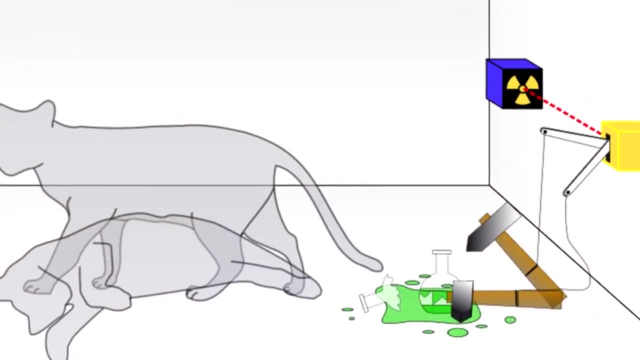 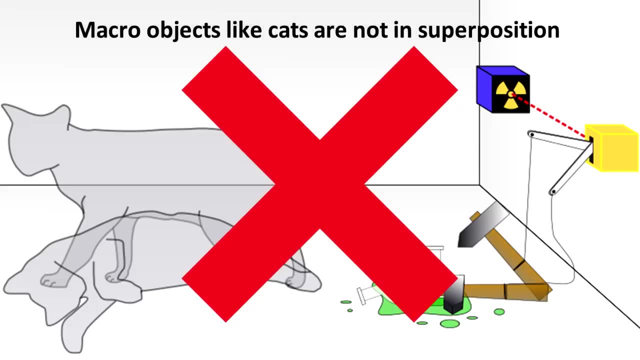 as you are going to get. This is the reason you and I and the cat in Schrodinger's experiment are not in superposition. The cat is not dead and alive at the same time. That's a myth And there is no possibility that the cat is dead and alive at the same time. That's a myth And there is no. 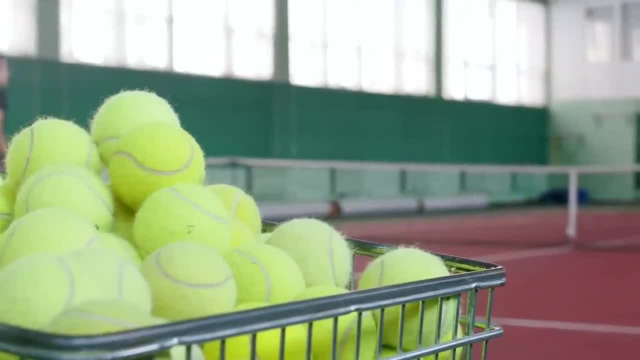 possibility that the cat is dead and alive at the same time. That's a myth. And there is no possibility that the cat is dead and alive at the same time. That's a myth. And there is no possibility of interference patterns being formed in our normal everyday interactions And for the same. 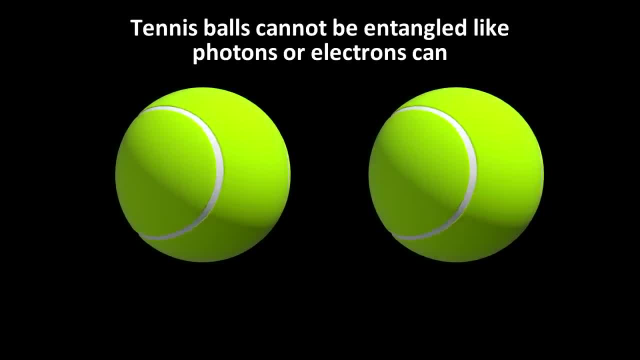 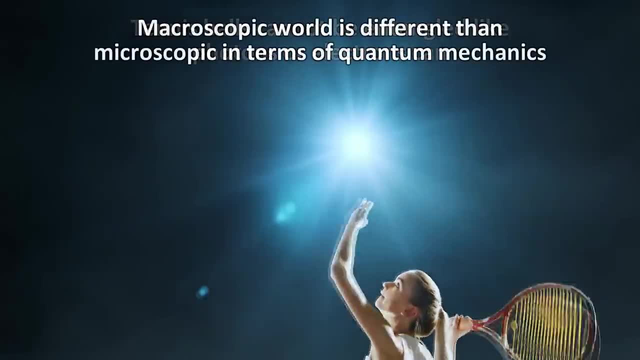 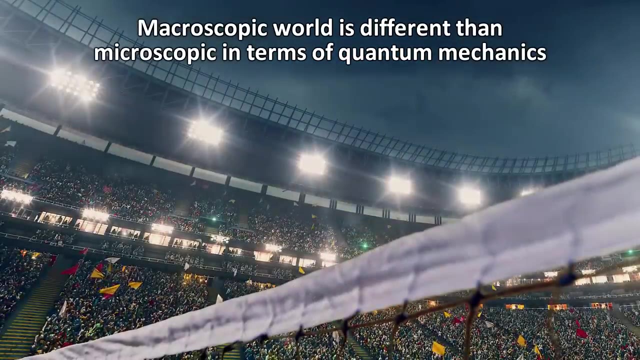 reasons, macroscopic objects like this cannot be entangled in the way photons can be entangled, for example. So what we see macroscopically is a very different world than what we see microscopically, And this is why it's a mistake to extrapolate our observations and equations.